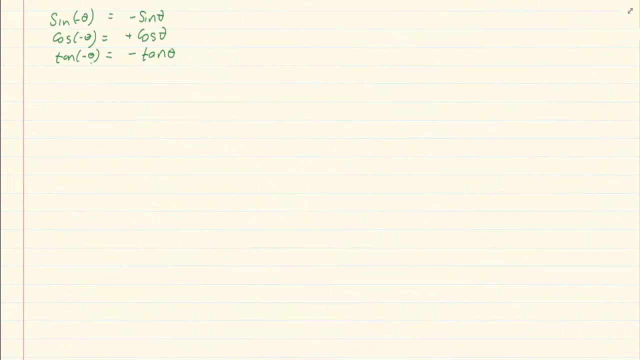 all fair and well, So sin negative theta becomes negative sin theta. Cause negative theta becomes positive cause theta and tan negative theta becomes negative tan theta. But in an exam, while you're stressed out and you can't really function, the best thing to remember is to simply add 360. 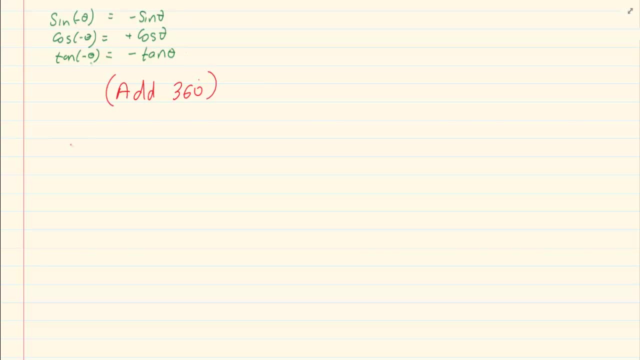 So if I give you sin negative 45 degrees, simply add a 360 degrees. So what do I have? I have sin 360 minus 45.. Do a reduction. It's in the fourth quadrant, so it's negative because I'm using 360. 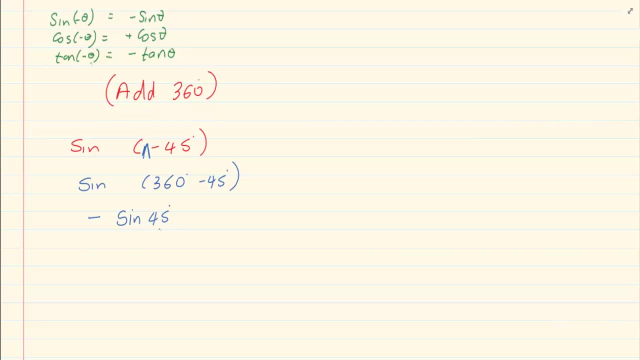 the ratio stays the same: 45.. Now, yes, it was easier to simply say, using these rules on top, that I could simply say: okay, so if it's a negative angle, as it is here, it simply becomes negative sin theta. I could have simply went on top said: okay, a sin, negative theta is negative sin 45, without doing the work of adding. 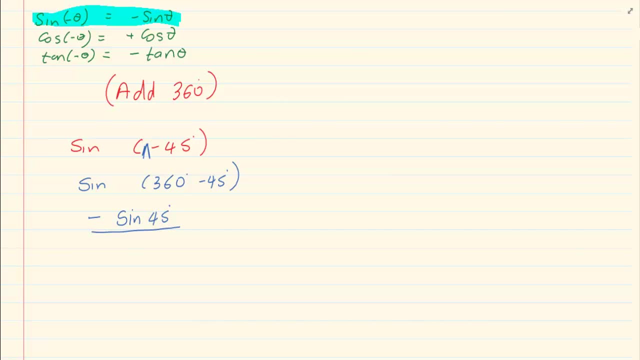 a 360. But what happens is Later pupils become confused. They end up with so many rules and so many methods to memorize that they can't remember all these rules. But add 360 is simply adding a revolution, which is something you learn when you're in like grade 7, when they do, a total revolution is 360 degrees. It is much easier. 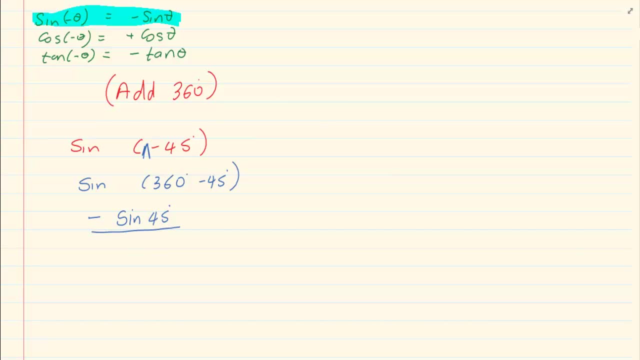 to remember. simply add a 360.. Let's do a reduction of cause negative 30. Now if I simply add my 360, I'm gonna have cause 360 minus 30 doing a reduction. it's in the fourth quadrant, so it's positive cause 30. Let's see how come the adding 360 becomes easier. What if I gave you the value? 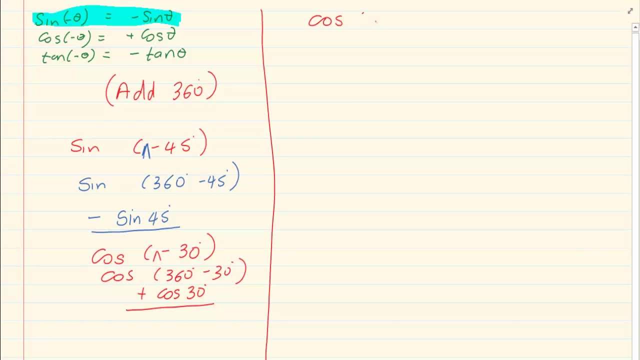 cause negative 225. Now, immediately you can look at this and you're gonna say, okay, this becomes cause 225. And then you do reduction, which is 180 plus 45, which then gives me minus cause 45. That's all fine. The problem is almost. 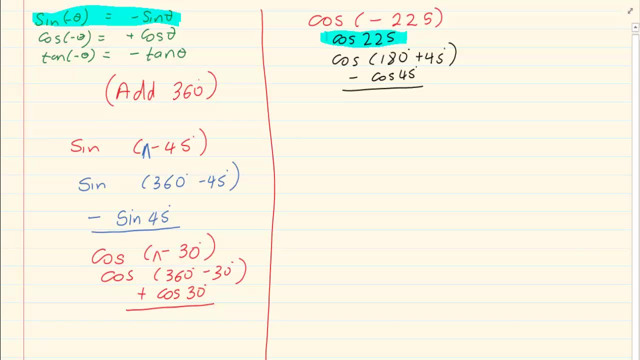 95. But 90% of the chance pupils write your negative cause 225. Common mistake repeatedly made. Now let's just add a 360. So I've got cause 360 minus 225. Which gives me cause of 135.. We know it's in the second quadrant. If I reduce I will get. 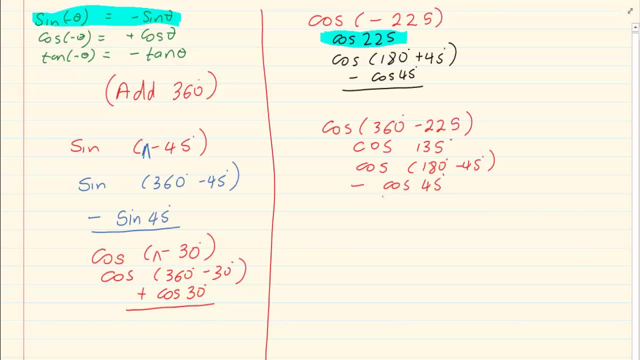 negative cos 45 degrees. So both methods you would get the same answer. But I am emphasizing that many times pupils make this mistake. Right another case where we would use the negative angle, where we would simply add a 360.. When the ratios are written upside. 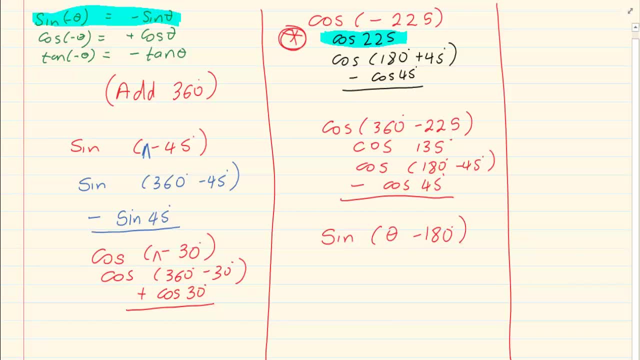 down. Theta minus 180 is not how we normally know it In our reduction. we know it as 180 minus theta. So we simply add 360 to this equation. And what would that give us? Sin minus 180 plus 360 gives me 180. And then my angle is positive, so it's plus theta. 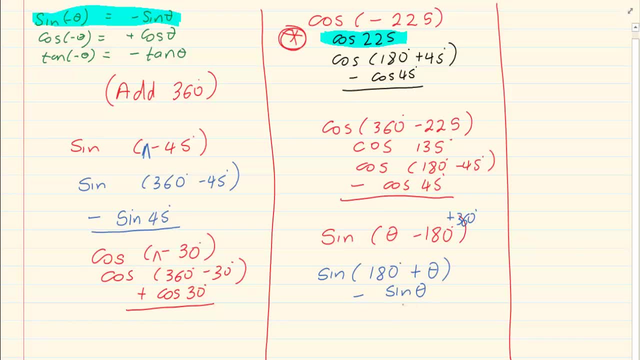 Reduce gives me negative Sin theta. Now, if you were trying to use the above rules, you would have taken out a negative, you would have swapped it and then you would have done a reduction of sin: 180 minus theta. The negative is there from your original that you have memorized, And you would still.